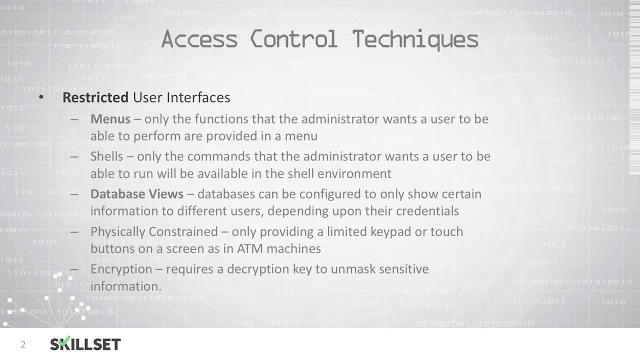 user may only be able to see three or four things. We can use shells to only allow certain commands that the administrator allows to be run in a shell environment. With databases we can use different views depending on who is accessing the system. In certain views we may provide additional. 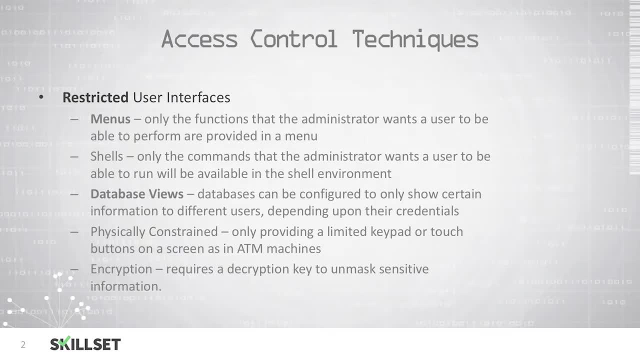 information such as a customer's social security number, but we would not allow all users to have access to that view. We can also physically constrain access to a system, such as on an ATM machine. there is only a keypad allowed to access the system. This is a great way to allow people to 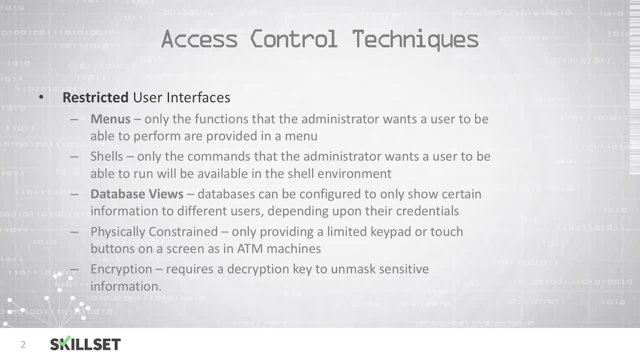 allowing the digits 0 through 9.. We are not allowing the users to enter data on a keyboard. We can also use encryption, which requires a decryption key in order to access sensitive information. We can control a user's access to information based on a content-dependent. 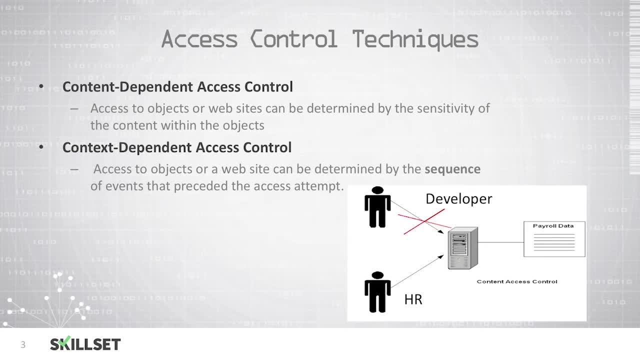 access control system or a context-dependent access control system. A content-dependent access control system restricts access to information based on the sensitivity of the information itself. For example, if we have top-secret data, we would not allow someone who only holds a secret security clearance to access that data. 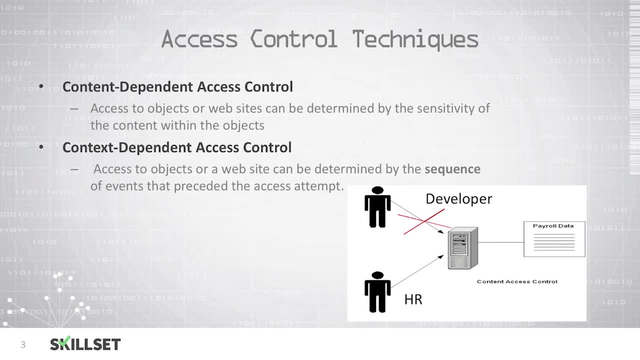 We can also place context-dependent controls in place. Here we're restricting the user based on the sequence of their events. For example, if a user attempts to access one piece of sensitive data, we may permit that, but if a user attempts to access three or 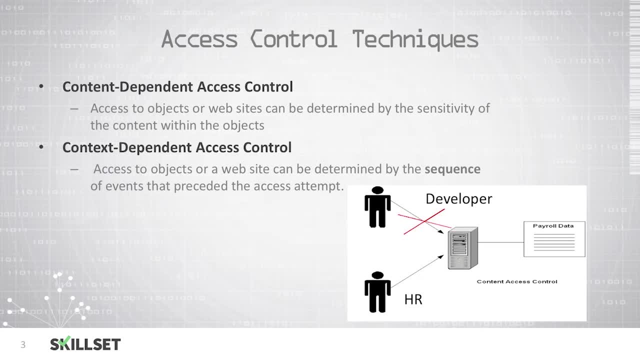 four sensitive pieces of data in a row, we may block them from accessing additional content. – or if a user attempts to access three or four sensitive pieces of data in a row, we may block them from accessing additional content – or if a user attempts to access. 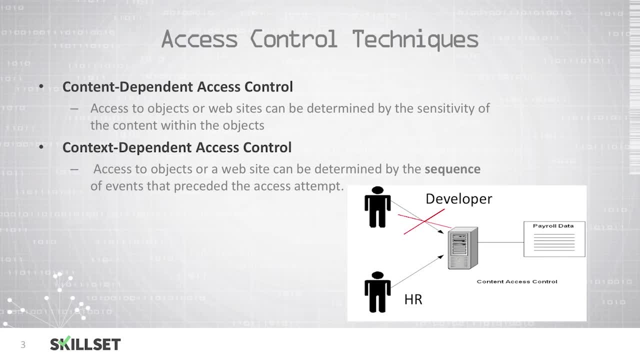 three or four sensitive pieces of data in a row, we may block them from accessing additional content. We can see at the picture at the bottom of the slide an example of content-based access control. Here we can see that an HR user is permitted to access payroll data. 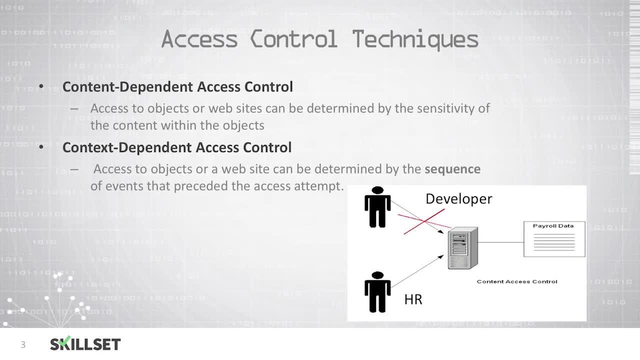 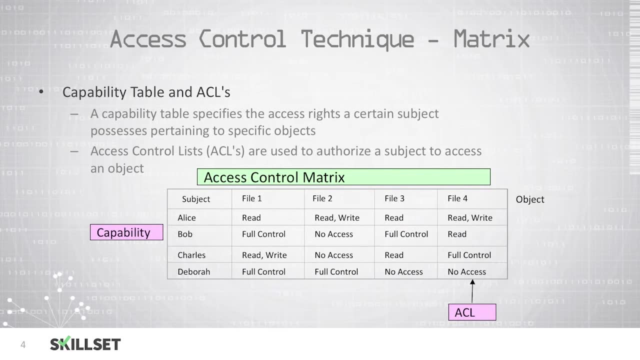 but someone from the development team is not permitted to access payroll data because that team should not have access to that information. We can use a matrix to maintain control of our resources and determine who has the ability to interact with them. A capability table specifies the rights that a user has when. 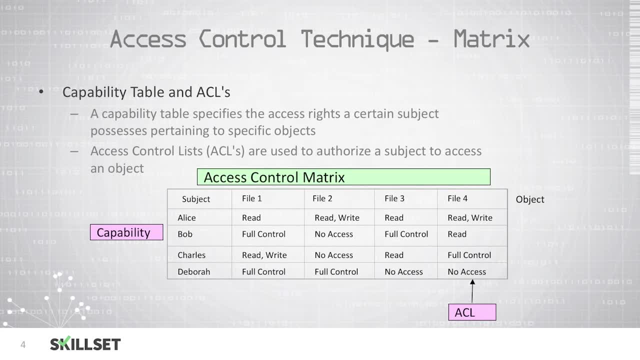 interacting with a certain object and an access control list is used to authorize a subject to access an object. We have an example of an access control matrix at the bottom of the slide. This tells us who has the ability to access which resources, For example, Bob.